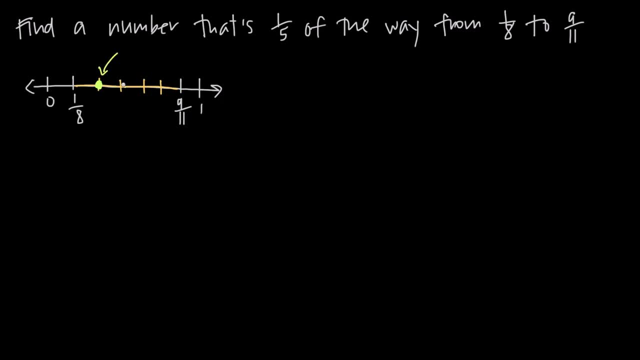 So we're interested in finding this number right here. Well, really, this number is just one-eighth plus one-fifth of however long this distance is. however long, the distance is between one-eighth and nine-elevenths. So the first thing we need to do is find out how long this section is. What's the distance between? 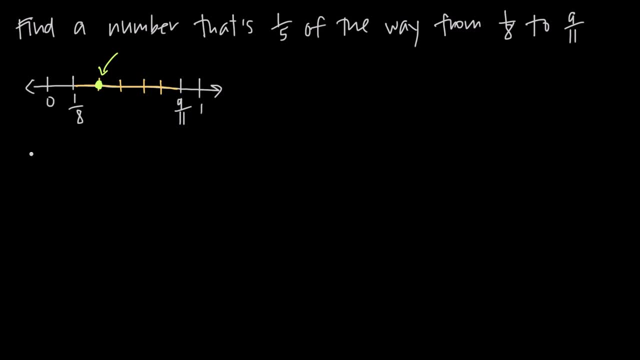 one-eighth and nine-elevenths. And the way that we're going to do that is we're going to say nine-elevenths, the larger number minus one-eighth, Just like if we wanted to find the distance between zero and one, we would take the larger number one and subtract zero. 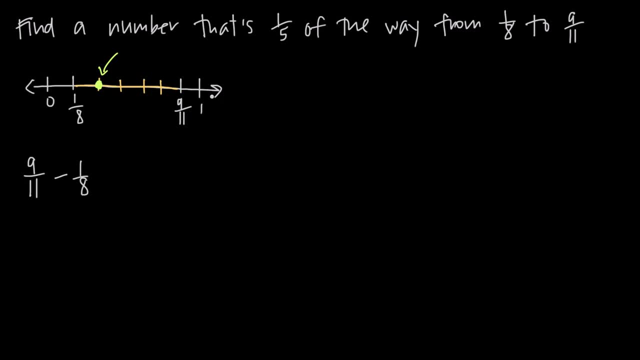 We'd say one minus zero is one. so the distance between zero and one on the number line is one Same thing here Between one-eighth and nine-elevenths. we take the larger number nine-elevenths and we subtract one-eighth to get the distance between them. 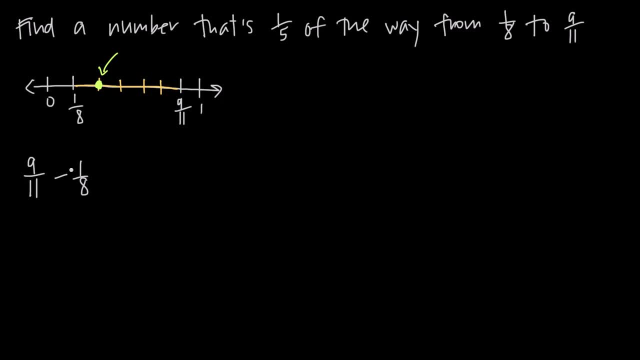 So now we just have a subtraction problem with fractions, which means we need to denominator is going to be 88.. So in order to get 88 for this first fraction, we're going to have to multiply by 8 over 8, so 8 over 8 times 9, 11th, to get 88 in the denominator. 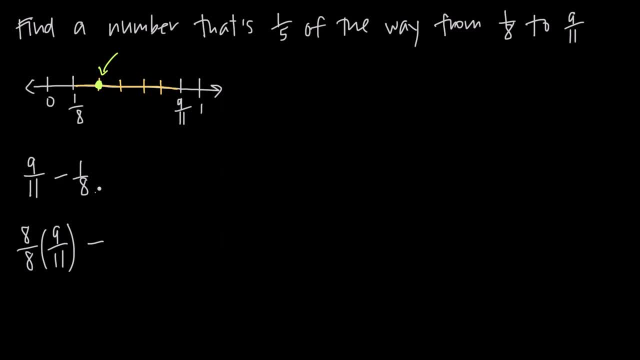 And to get 88 in the denominator of 1: 8th we're going to have to multiply by 11, over 11 times 1, 8th, like this: And now, when we do our multiplication 8 times 9 is 72 over. 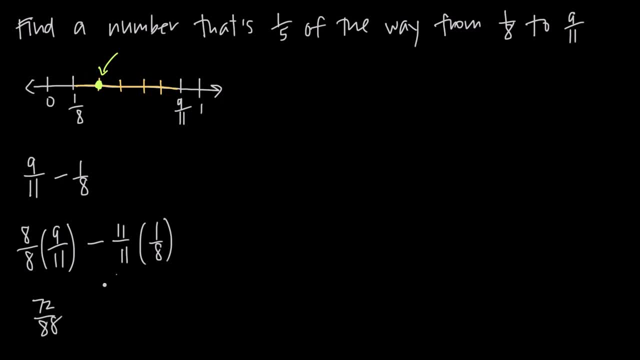 88.. 11 times 1 is 11,. so minus 11 over 88. And when we do 72 minus 11, we get 61. So 61 over 88 is the distance between 1 8th and 9 11ths. So the length of this orange section. 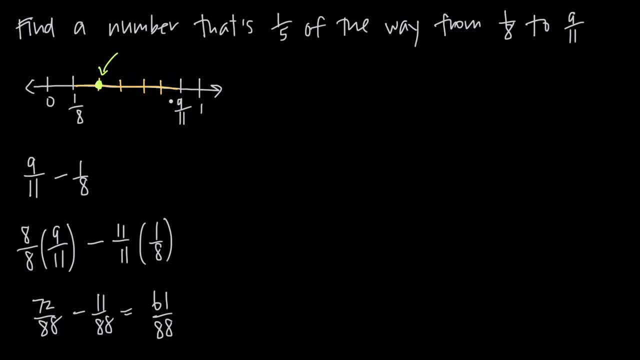 here is 61, 88ths. Now we need to find the length of just 1, 5th of this distance. So in other words, we found the length of the orange section, but now we need to find the length of 1, 5th of it to get this length right here. So we're going to have to multiply by 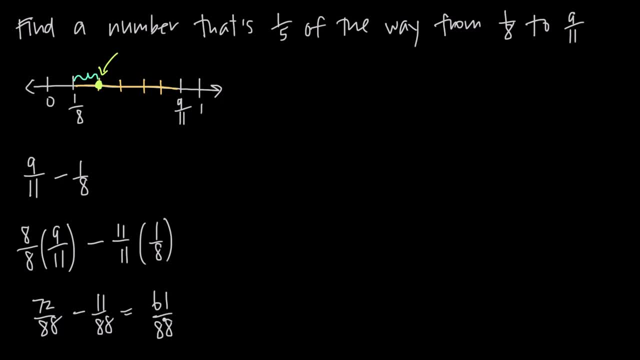 8 times 9 is 72 over 88. So in order to find the length of 1- 5th of it, we just have to multiply by 1- 5th or divide this thing by 5.. Remember, dividing by 5 is the same as multiplying by 1- 5th. So either 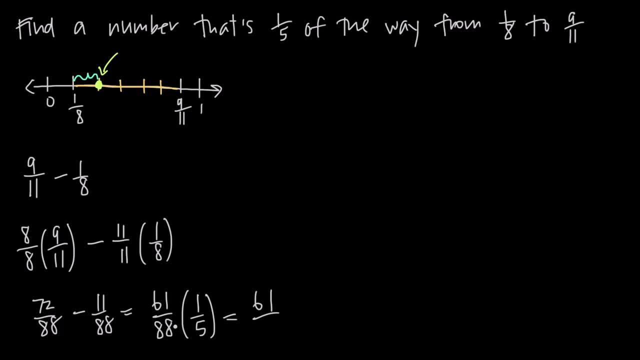 way, when we multiply across, we're going to get 61 over 88 times 5 is 440.. So that tells us that the length of this particular section right here, this length, the distance between 1, 8th and this point that we're interested in, is 61 over 440. 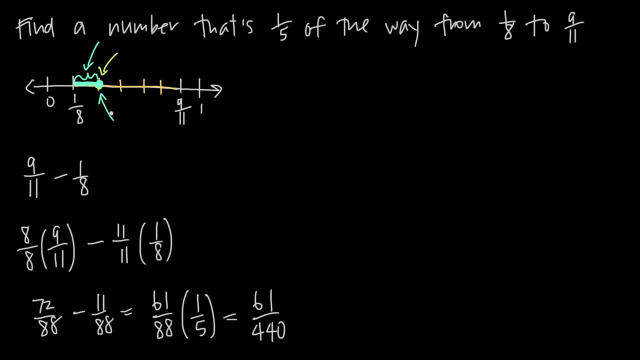 So now, in order to find this exact point right here, we need to do 1 8th plus 61 over 440.. Because if we do 1 8th plus 61 over 440 on the number line, that'll land us right at. 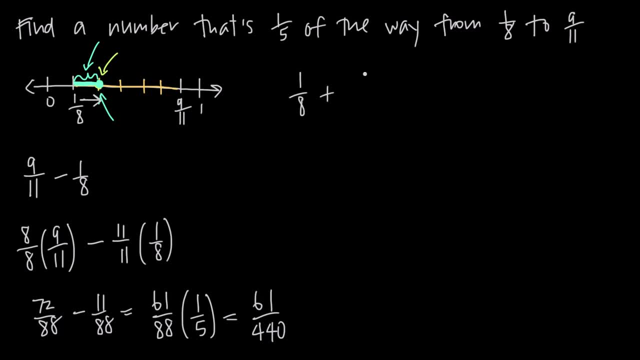 this point that we're interested in. So we'll do 1: 8th plus 61 over 440.. We need to find a common denominator and we can find a common denominator of 440 if we multiply this first fraction by 55 over 55.. 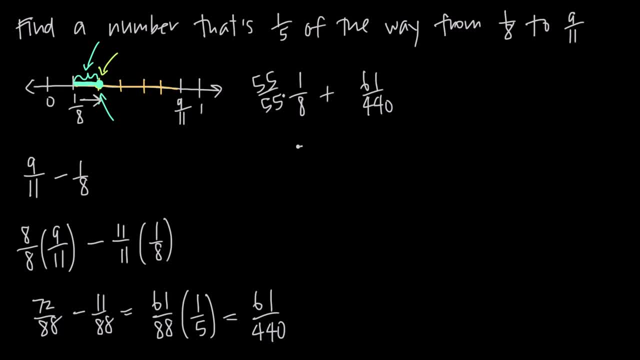 So this is 1 8th plus 61 over 440.. So 1 8th plus 61 over 440 is 440.. So multiplying across here 55 times 1, we have 55.. 55 times 8 is 440.. Then we add 61 over 440.. 55 plus 61 is. 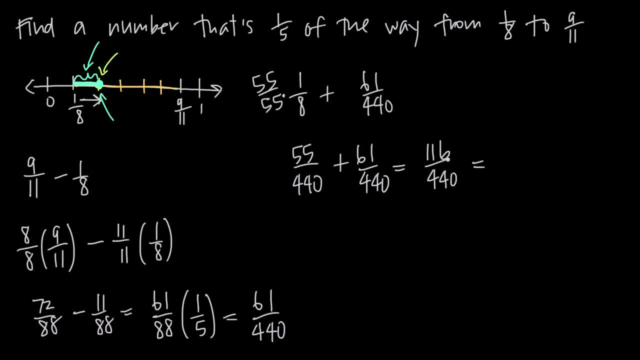 116 and, of course, our common denominator of 440.. Now we can divide both the numerator and the denominator by 2.. We want to reduce the fraction as much as we can. Because both the numerator and denominator are even, we'll divide by 2.. 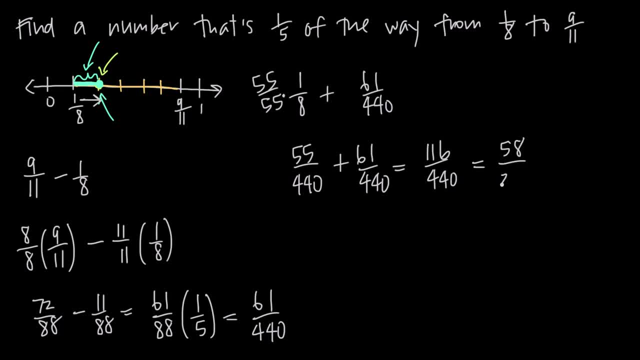 So 1, 8th plus 61 over 440 is 58.. 440 divided by 2 is 220.. We have even numbers still, so we can divide by 2. again, 58 divided by 2 will be 29.. And 220 divided by 2 will be 110. 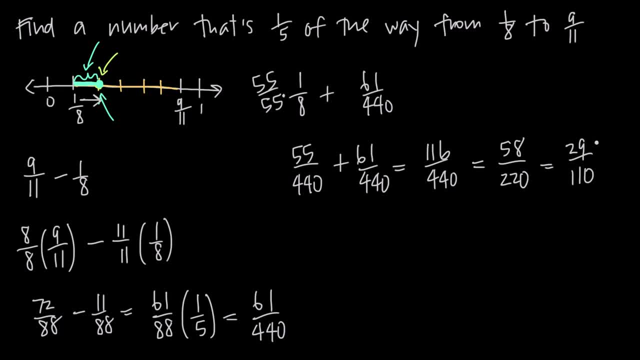 29 is a prime number. It has no factors other than 29 or 1.. And 29 doesn't go evenly into 110.. So this is now an irreducible fraction. We've reduced it as much as we can, which means this will be our final answer. So if we were going to label this point right here, 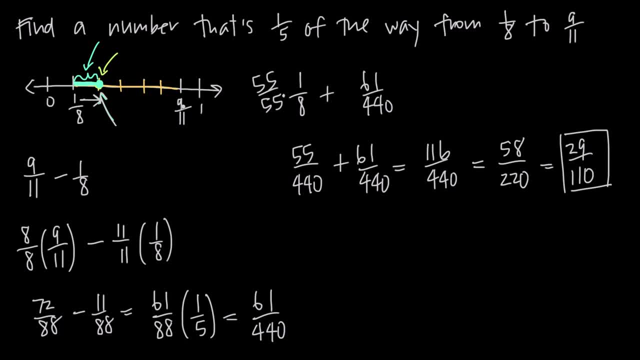 just like we labeled this point on the number line as 0,, this one is 1, 8th, this one is 9, 11ths. If we were going to label this point, we would label it as 29 over 110. And we know. 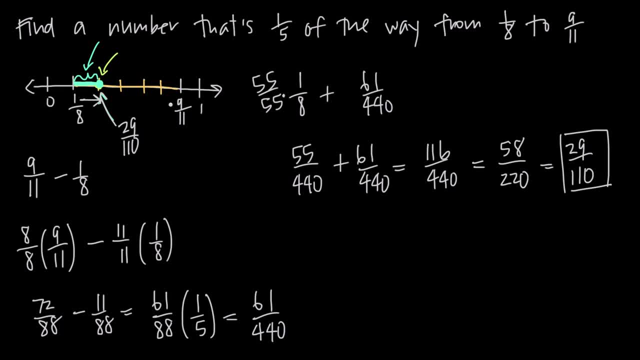 that that point is 1, 5th of the way from 1, 8th to 9, 11ths.